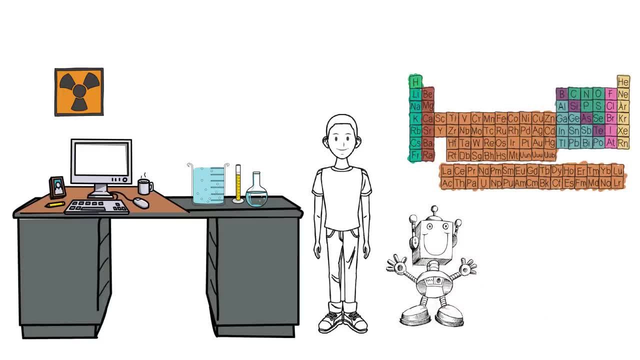 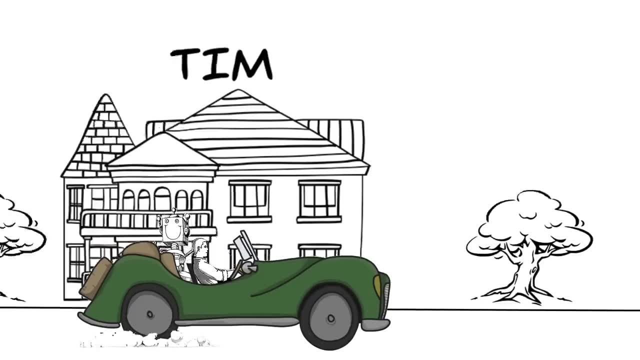 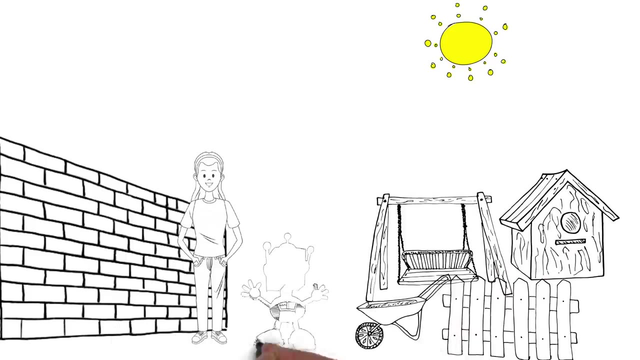 Meet Tim. Tim builds a robot in his lab- A climate-controlled and pollution-free environment. Once he's done, he drops the robot off at his project partner, Mia's house. Mia takes it out to her backyard to ensure that the robot meets the requirements. But here is where the problem. 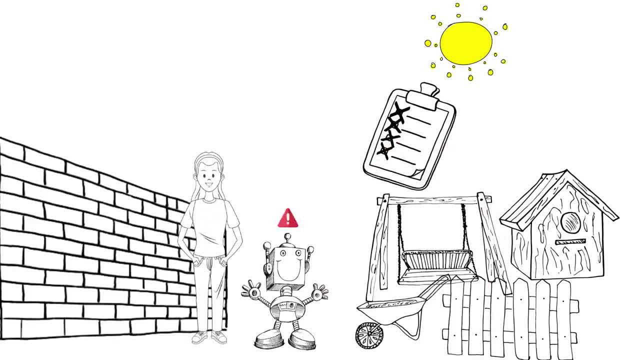 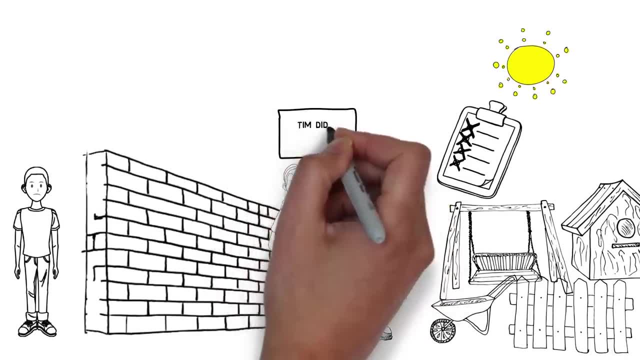 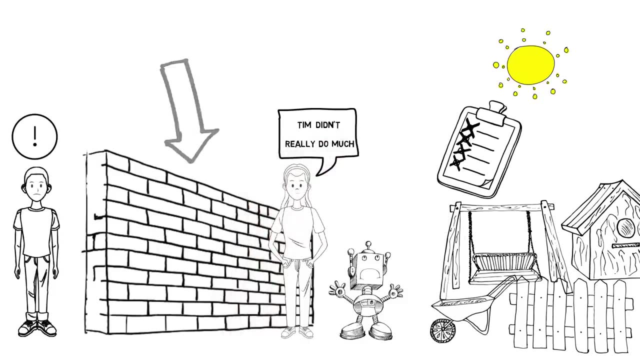 arises, The change in the environment causes the robot to malfunction. Mia is now really annoyed and she has a lot to correct, And it seems to her as though Tim didn't really do much. This wall between them leaves the poor robot to bite the dust. Well, what if we broke this wall? 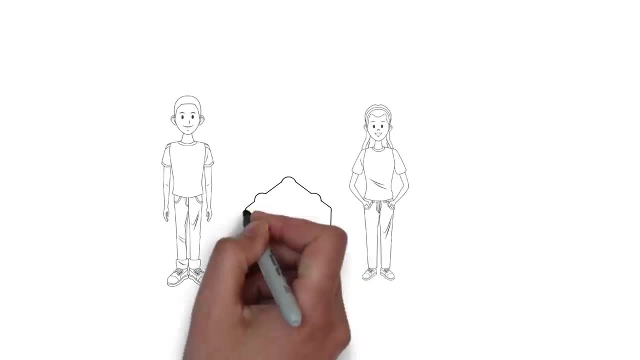 Tim and Mia now work together in a common space. Tim develops each block of functionality of the robot, which is then immediately checked by Mia. Both are now working simultaneously instead of waiting on the other to finish their task. As and when a feature is ready, the robot will. 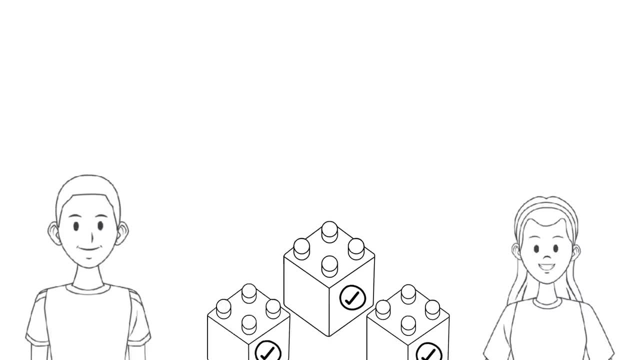 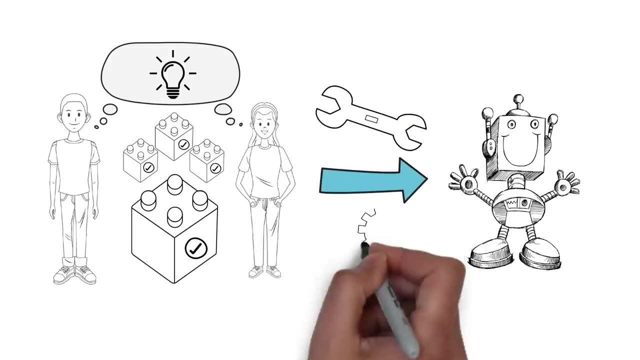 be your final product. They only for use. they are put together to build the final product. They develop a common mindset and share ideas. To further speed up the process, they use several tools which can automate every stage. This means that the robot is now ready sooner. 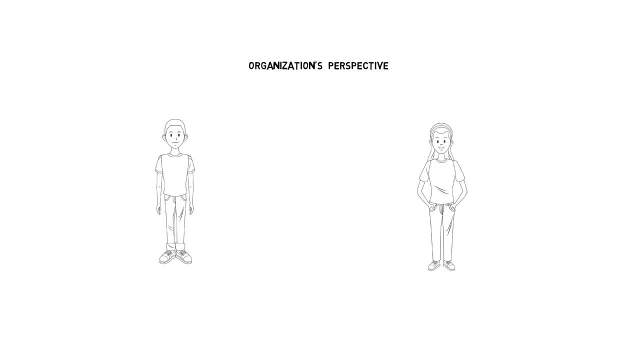 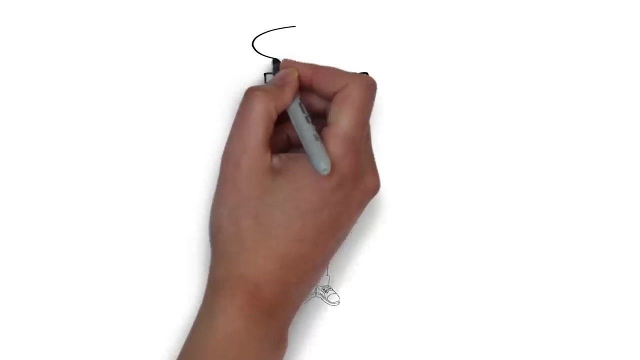 with less iterations and manual work. From an organisation perspective, Tim would be the developer, while Mia the operations. Their union is the core of the DevOps approach and set of tools to automate each of these stages. Let's have a look at these. 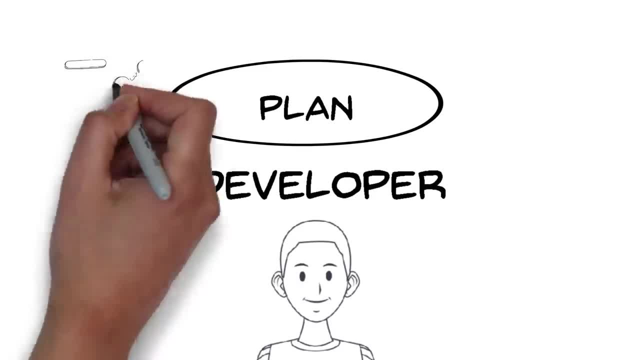 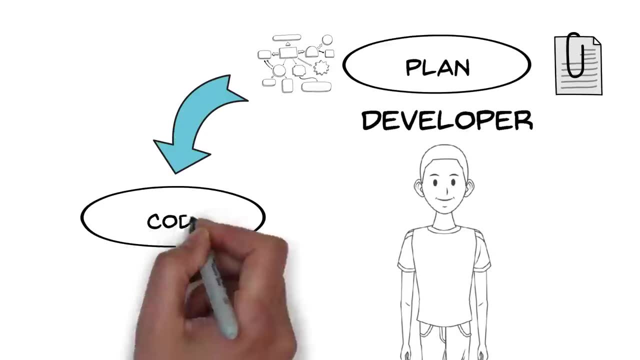 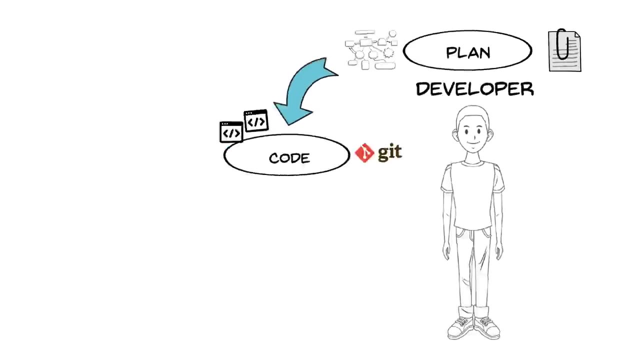 Tim first puts down a plan. In terms of a software, this could mean deciding on the modules and the algorithms to use. Once he has the plan, he now codes the plan With tools such as Git. Tim has a repository for storing all the codes and their different versions. 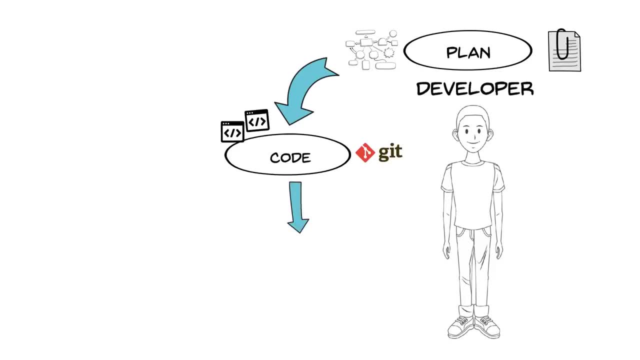 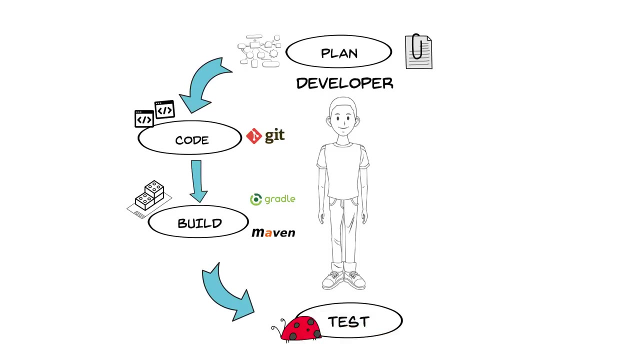 This is called version control. Next, this code is fetched and made executable. This is the build stage. Tools such as Gradle and Maven will sort this out. Now, before deployment, the product is tested to catch any bugs. The most popular tool automating testing is Selenium. 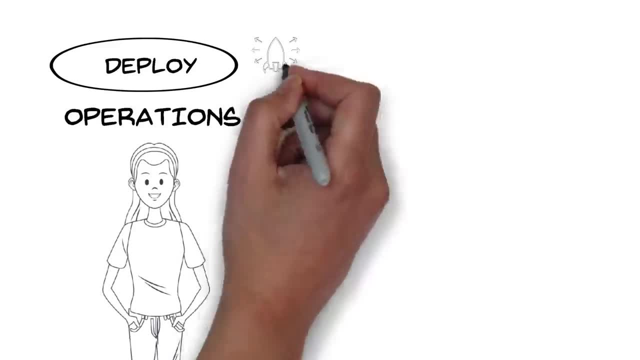 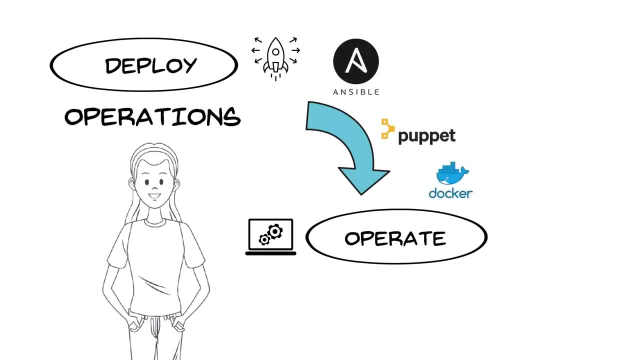 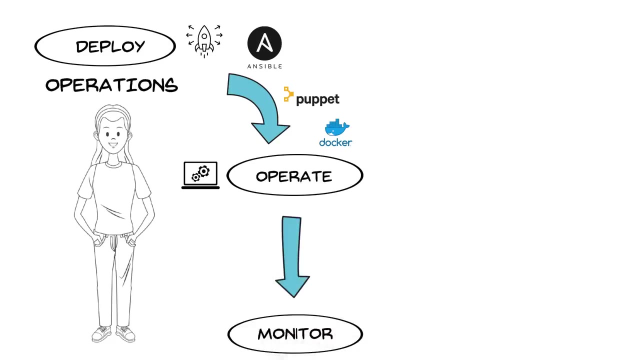 Once the products are tested, Mia must deploy it. The deployed product is then continuously configured to the desired state. Ansible Puppet and Docker are some of the most common tools used that automate these stages. Now every product is configured, It is continuously monitored in its working environment.